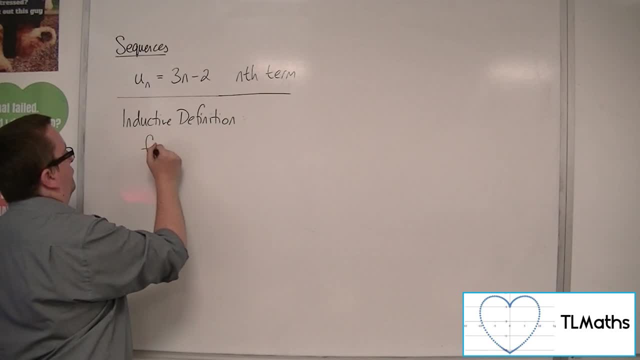 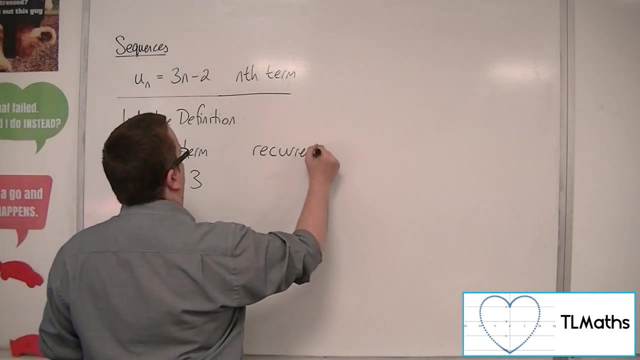 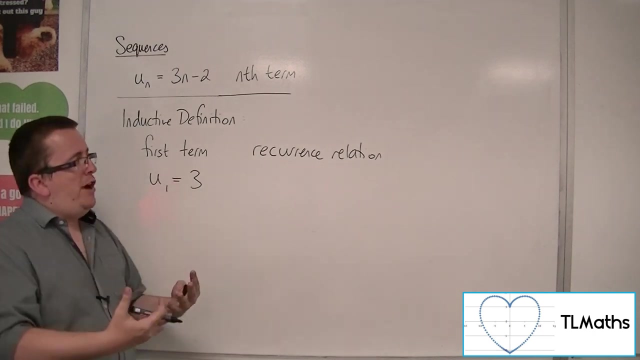 A first term, Okay, which we will say is u1, which might be equal to 3,, for example, And a recurrence relation. Now, the recurrence relation is an instruction and tells you how to get to the next term. So if we say that the current term is u1.. 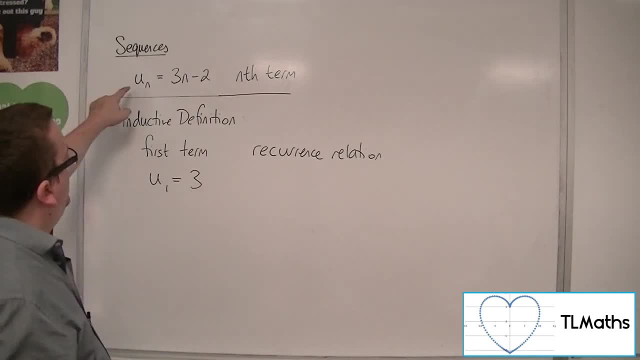 So if we say that the current term is u1.. Okay, now I know we're using u1 up here as the nth term and we're kind of using it here as well. So for the nth term that we get to, okay in the sequence. 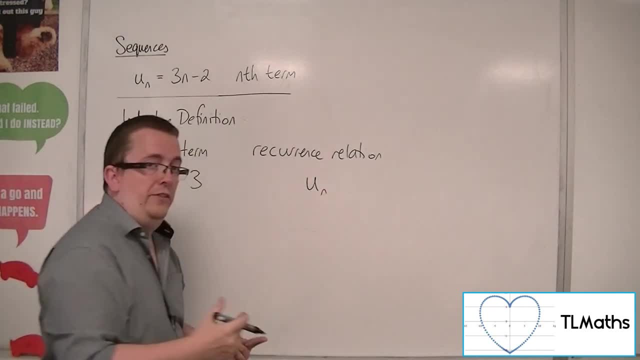 So let's say this is my nth term, the nth term in the sequence that I've arrived at. I'm going to multiply whatever that value is by 2, and then subtract 3,, and that will give me the next term in the sequence. 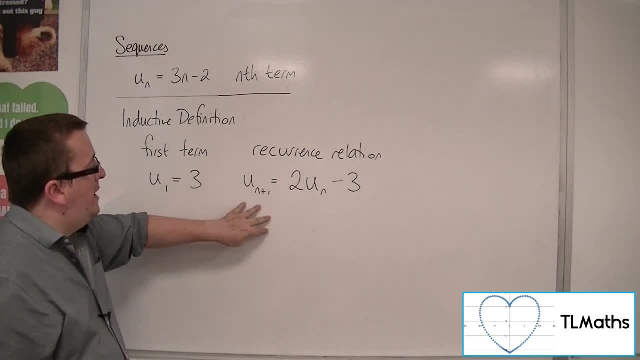 I'm going to multiply whatever that value is by 2, and then subtract 3, and that will give me the next term in the sequence. So the next term in the sequence- un plus 1, is 2. lots of the previous term, take away 3.. 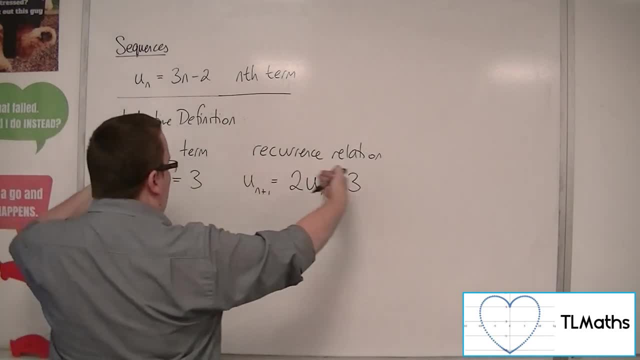 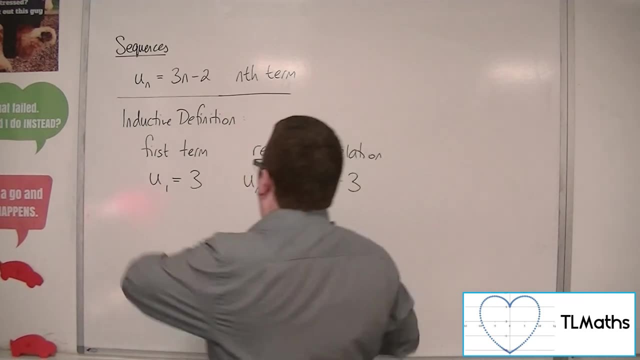 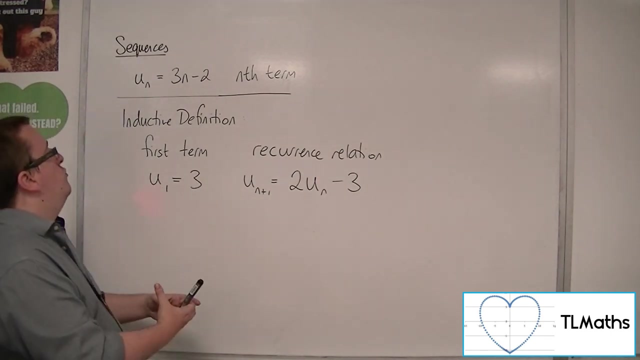 That is what that is saying. And this together is an inductive definition, Because just by itself, that bit or that bit, neither of those, give you a sequence. You need both pieces to create this inductive definition. Okay. 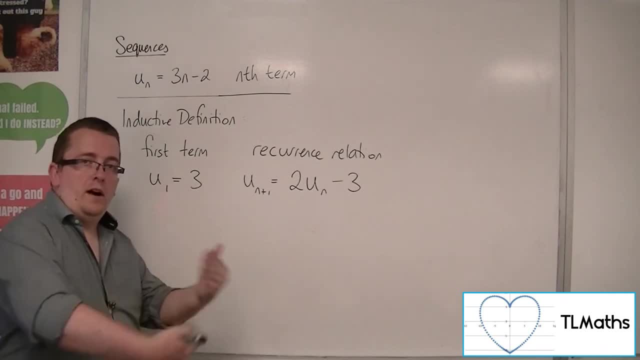 So this word inductive means one after the other, And this is what we refer to as a term-to-term rule, term-by-term rule. Okay, Because I need the previous term to know what the next term is. Okay, And so from that you can go right. well, the next term- u2, will be 2, lots of the previous term, take away 3.. 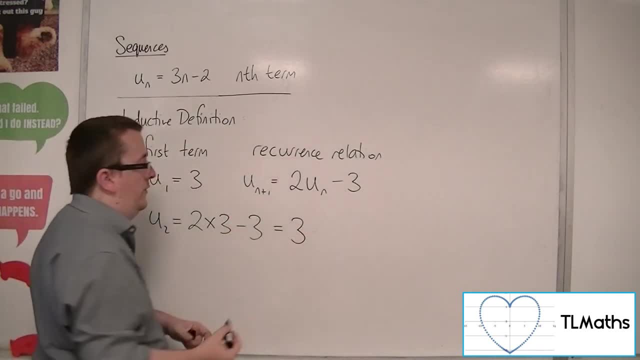 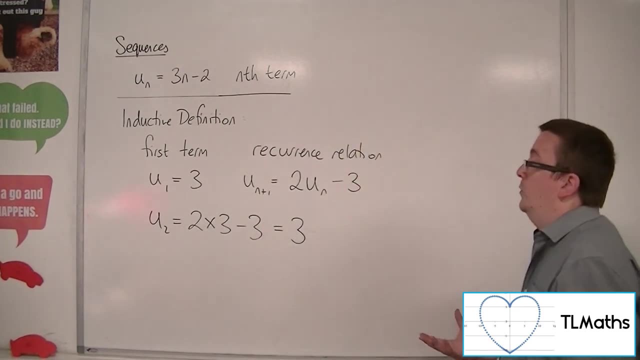 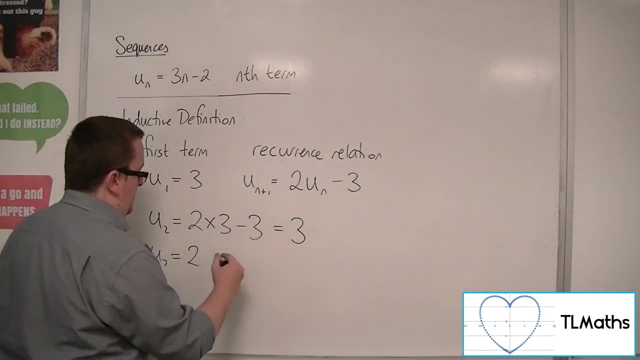 So 6,. take away 3,. oh, that's 3 as well, It just so happens. Okay, Now this sequence here as you work through right. so u3 would be 2, lots of the previous term. take away 3, which is 3 again.